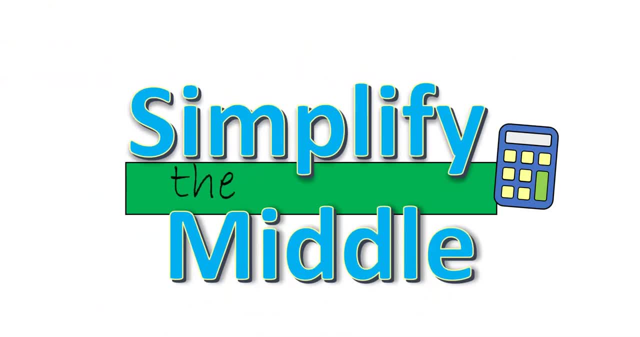 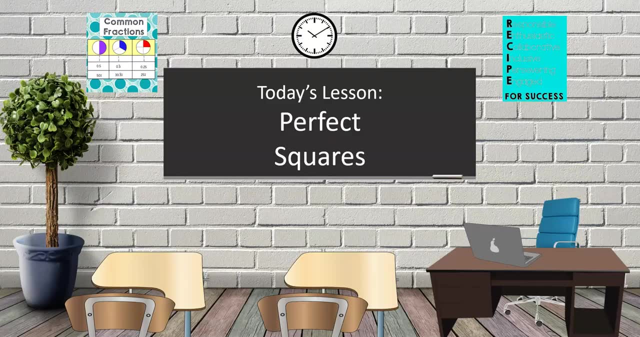 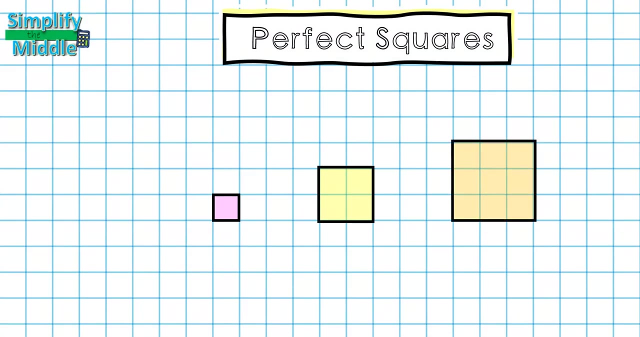 Hi and welcome to today's lesson: perfect squares. Take a look at the following quadrilaterals. We know that these are all squares because they have the same length and width. Let's take a closer look at what it means to be a perfect square. If we look at the pink square, we notice. 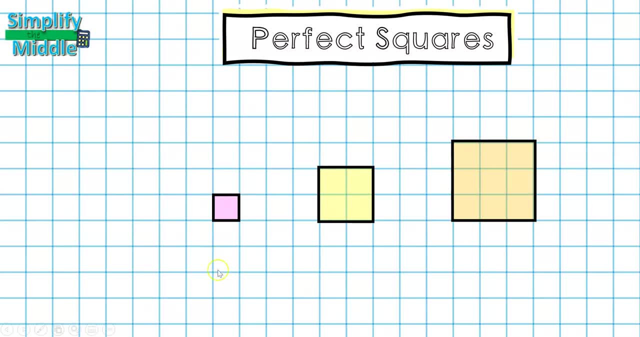 that the length is 1 and the width is 1.. We also notice inside the square there is one box, so 1 would describe the perfect square here. On the yellow square we have a length of 2 and a width of 2 as well, So we know that we can see a total of 4 boxes inside this square, so 4 is our perfect. 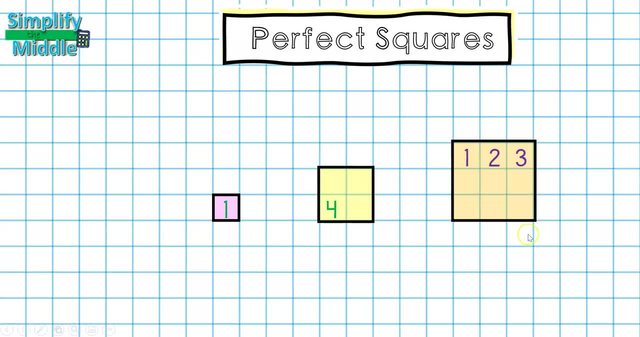 square Over here on our orange box we've already counted out a length of 3 and we see we also have a width of 3.. Inside this square we can see that we have 1,, 2,, 3,, 4,, 5,, 6,, 7,, 8, 9 boxes. So here 9 is. 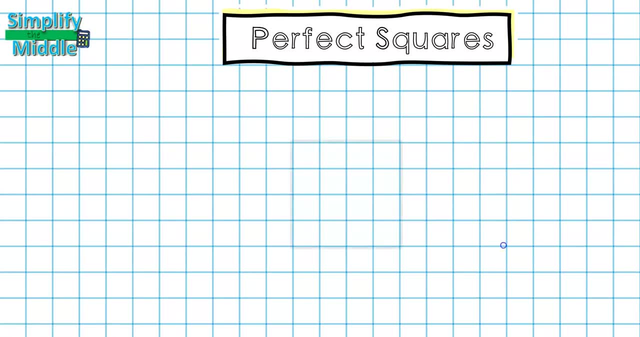 our perfect square. Following this pattern, we can easily see that perfect squares mean the amount of boxes inside a square. Here's another square. Take a moment to see if you can find the perfect square. I see that this square has a length of 4 and a width of 4.. Because it has the same length and 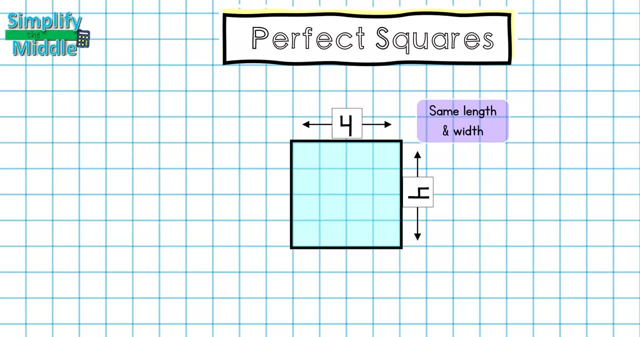 width. I know that the number of boxes on the inside are going to be 4 times itself, So 16 is going to represent our perfect square. Let's look at perfect squares in relation to exponents. If I'm counting the length of this square, I see that it has a side length of 6 and it has a width of 6 as well. 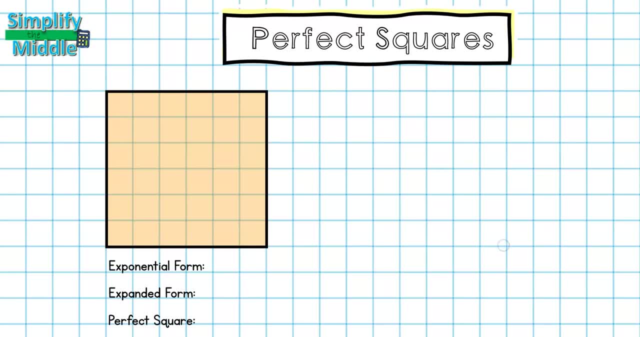 We can write this in expanded form as 6 times itself, 6 times 6.. Because it has been repeated twice, I know that the exponent here is going to be 2, and the base is going to be 6.. So this is 6 squared. 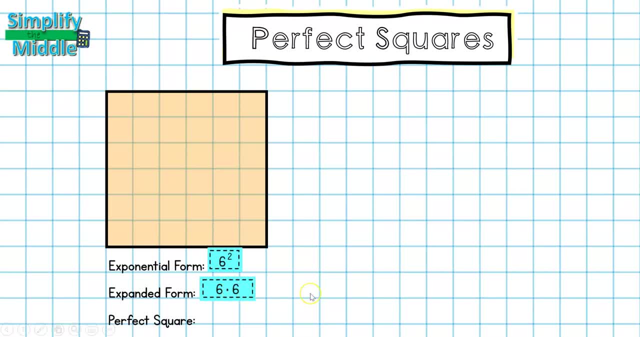 And if I were to multiply together 6 times 6 to find the area, I would see that I have a perfect square of 36.. Now you try Pause the video and see if you can find the exponential expanded in standard form of this square. 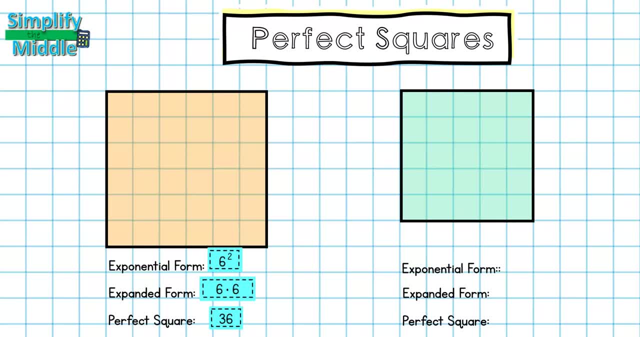 You should have counted a length of five going across and five going up and down. That would give you an expanded form of five times five. Because I have a base of five and I've repeated the five twice, my exponential form will be five squared. 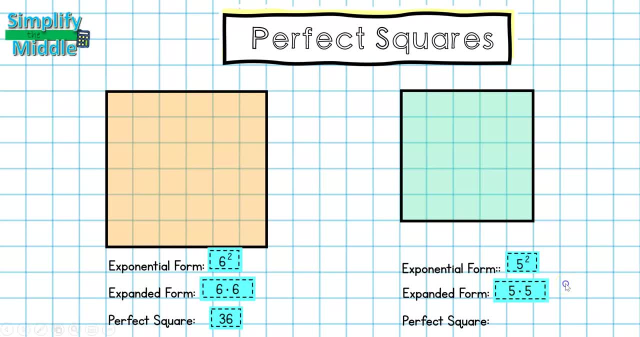 And finally, when I multiply my fives together, I get 25.. So 25 is another example of a perfect square. Notice that all of the squares that we got- 1,, 4,, 9,, 16,, 36,, 25, are all representing. 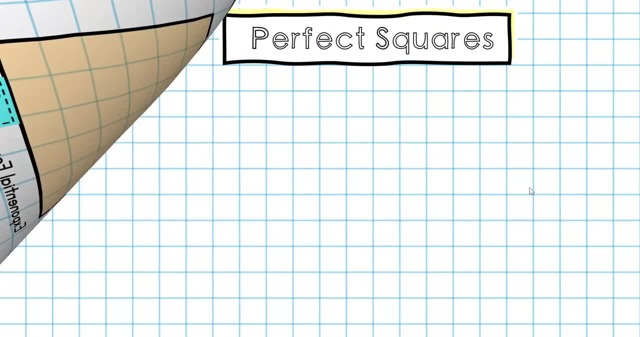 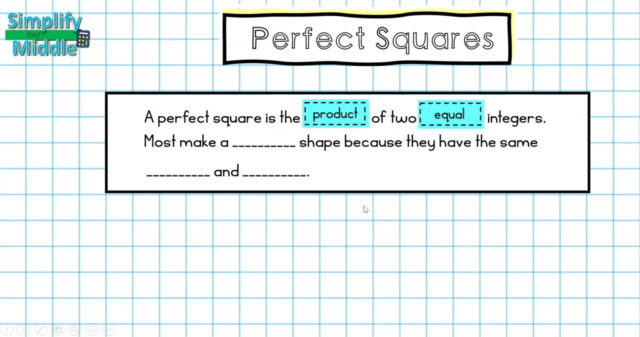 the area of a square shape. Let's recap: A perfect square is the product of two. Most will make a square shape because they have the same width and length. Notice how we talked about 1,, 4,, 9,, 16,, 25, and 36.. 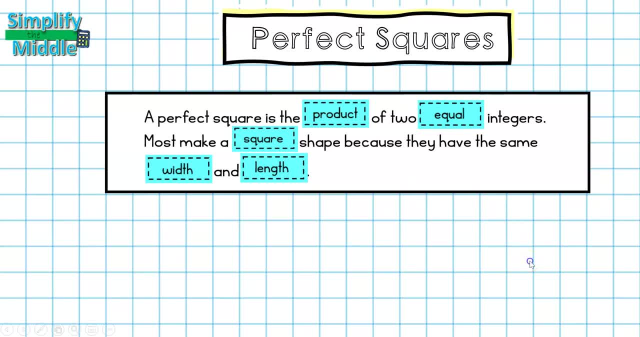 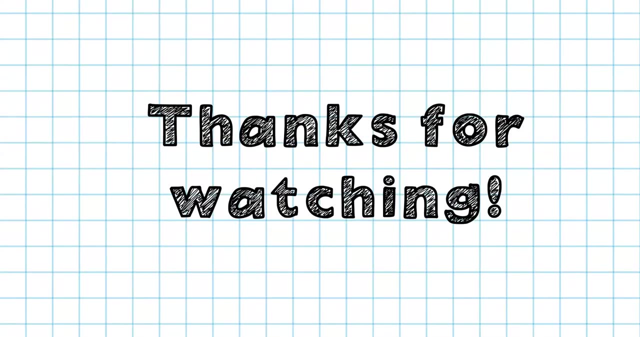 There is one more perfect square that does not make a square at all, though, And this is zero. So, even though it does not make a square, zero is a perfect square, because zero times itself is zero. That wraps up our lesson. Thanks so much for watching. 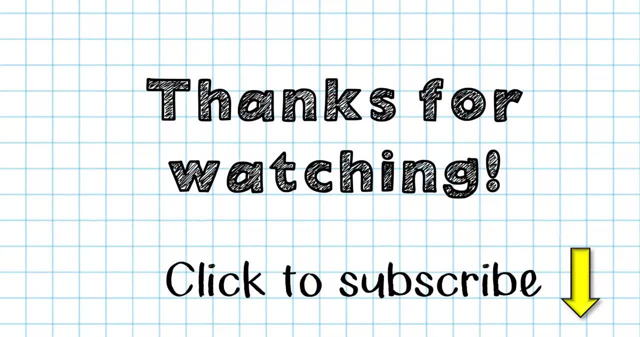 Feel free to click the red subscribe button so you'll always have access to this and other lessons. Thanks again for tuning in, Until next time.